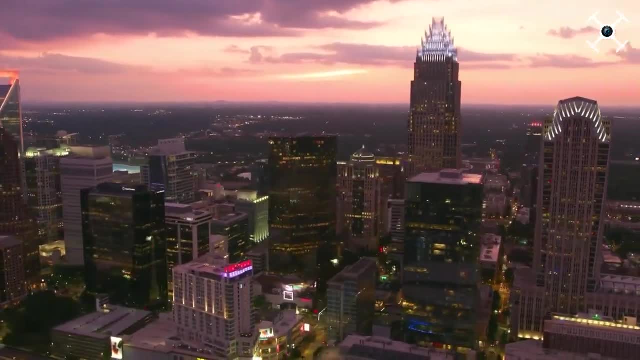 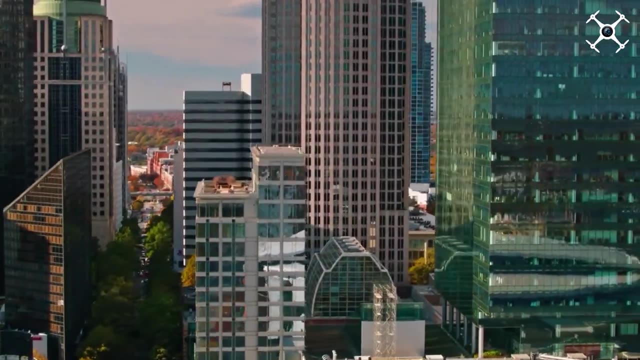 offer to all income levels and, surprisingly, it is actually extremely affordable. If you ask any North Carolinian, they will say, hands down, that North Carolina is one of the best states in the country And in order to be one of the best, 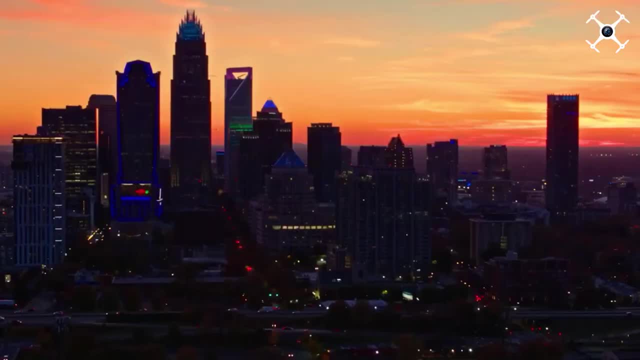 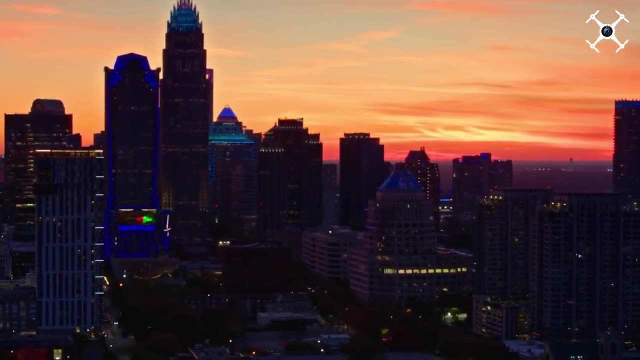 they have to have some of the nicest, most affordable places to call home right. If you're set on an exciting new city that'll give you the best bang for your buck, you have to check out these top 10 most affordable cities the old North State has to offer. 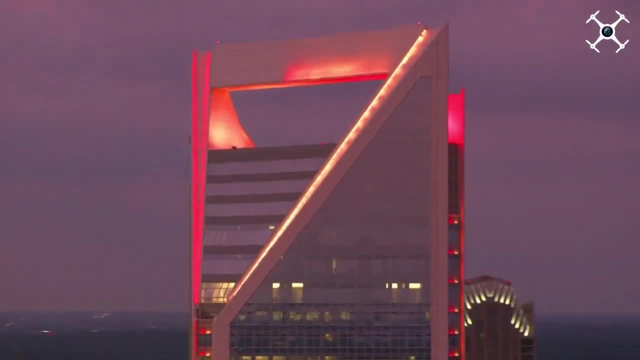 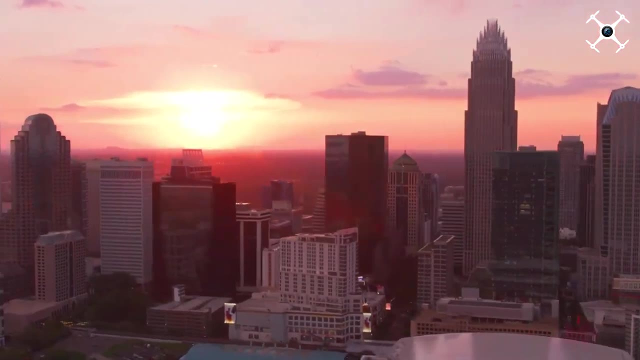 Kindly make sure to hit the subscribe button and press the bell icon before we start this video about the 10 most affordable places to live in North Carolina. Now let's dig deeper into each of the top 10 most affordable cities in North Carolina. 10. Ashboro. Home to one of the world's largest natural habitat zoos, Ashboro is an affordable and family-friendly community to reside in. With over 25,000 residents, Ashboro isn't quite a small town, but doesn't have the noise and crowds of a big city either. The recently renovated mall. 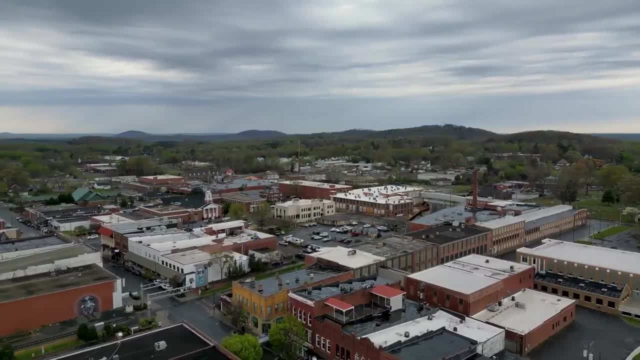 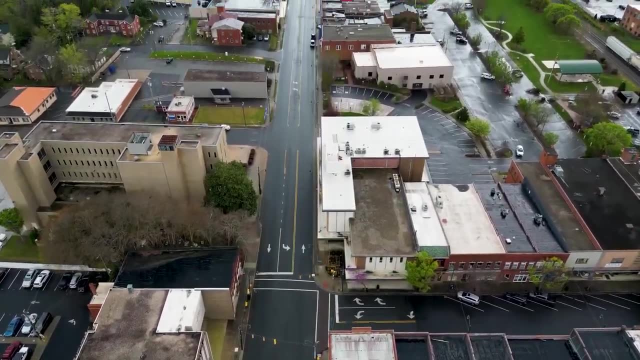 charming downtown district and well-kept neighborhoods provide the perfect backdrop for suburban living. However, if you want a little more excitement, Ashboro is close enough to beautiful beaches, mountains and multiple cities for a leisurely day trip Like Reidsville, a majority of Ashboro 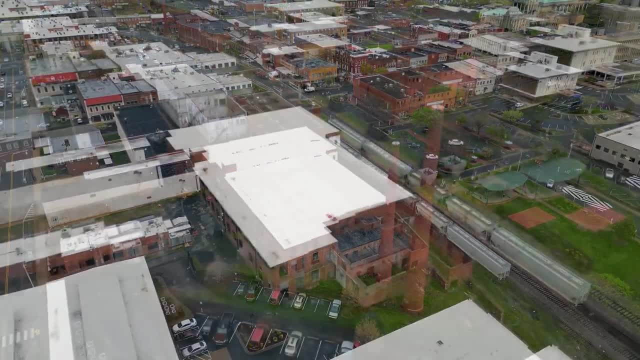 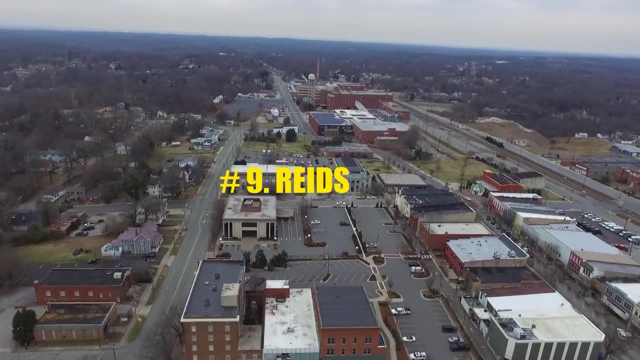 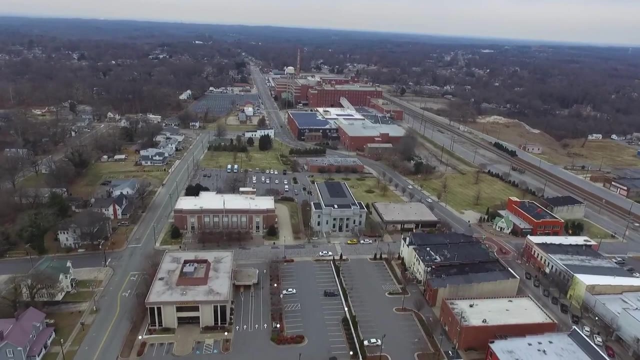 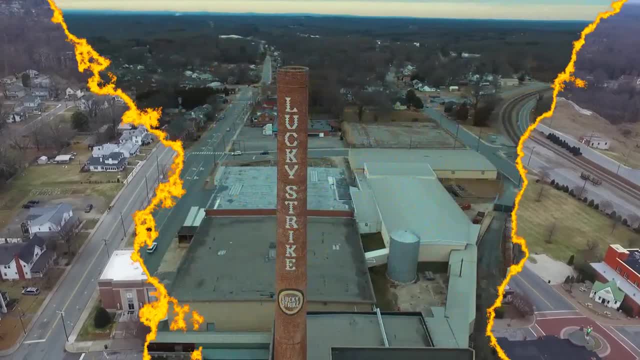 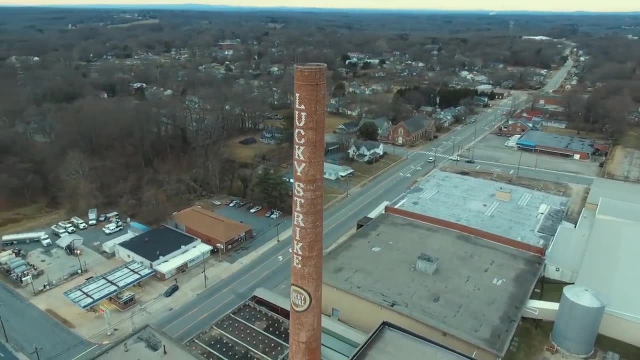 This sleeper city has plenty to offer newly married house hunters and young professionals in the way of outdoor activities, museums, art galleries, farmers' markets and historic attractions. And if you're craving a night on the town, Greensboro is less than a half-hour drive. 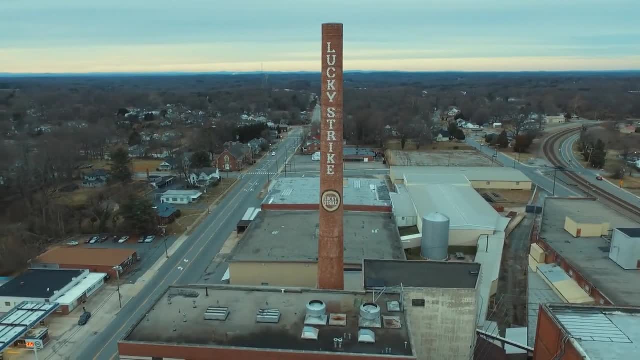 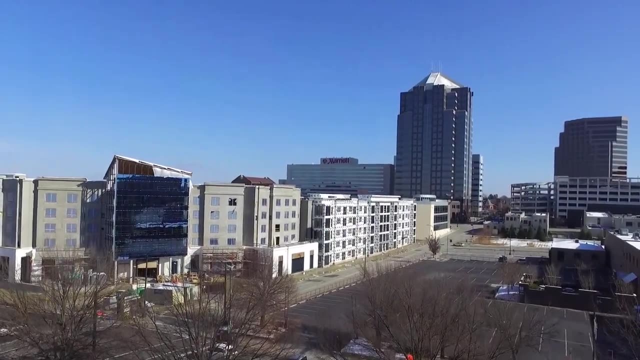 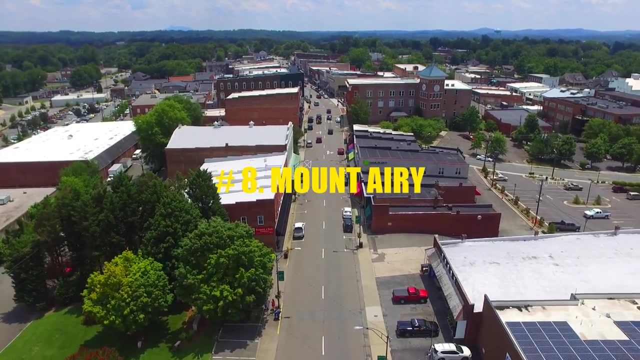 Many young people who live in Reidsville commute to Greensboro for work, so there are plenty of opportunities for residents looking to advance their careers while saving some serious cash on living expenses. Number 8. Mount Airy. Located in Yadkin Valley, North Carolina's wine country, Mount Airy is a hub for wine and beer. 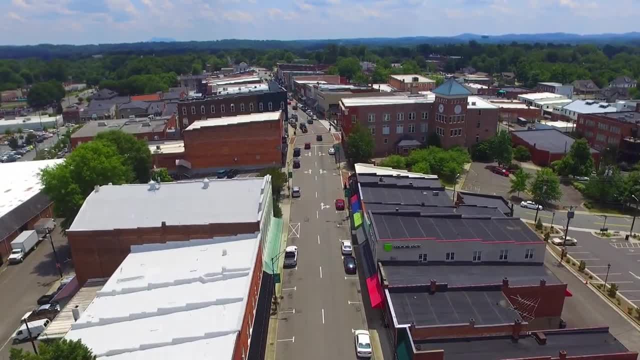 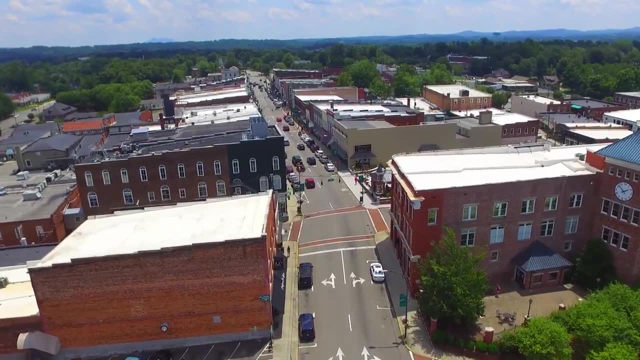 enthusiasts. However, fans of The Andy Griffith Show may be more familiar with the town's main attraction, Mayberry, With storefronts like Floyd City Barbershop and Snappy Lunch. a stroll down Main Street in the friendly city transports you straight into the endearing 60s TV series. 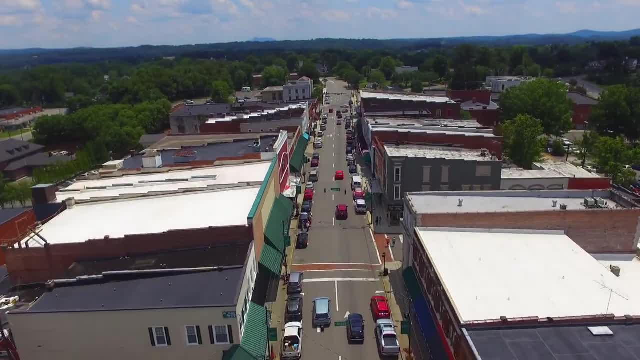 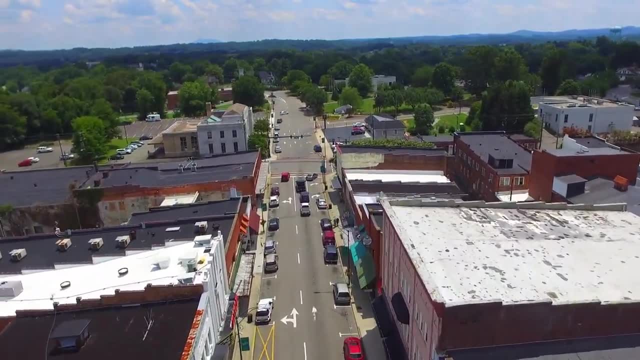 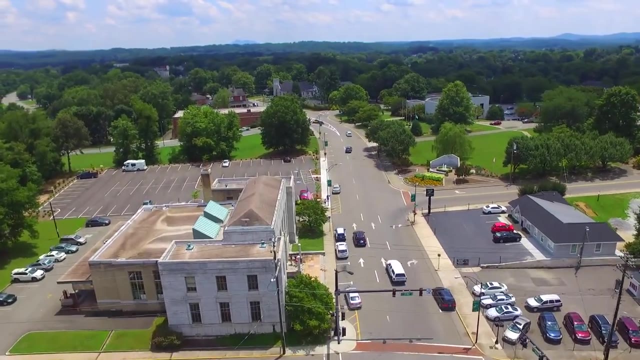 The nostalgic atmosphere and low-cost living makes Mount Airy one of the best places to retire in North Carolina. The city is committed to providing more age-friendly resources so elderly residents can participate in community activities. However, anyone looking to step away from the hustle and bustle of city life will find plenty to enjoy in Mount Airy. 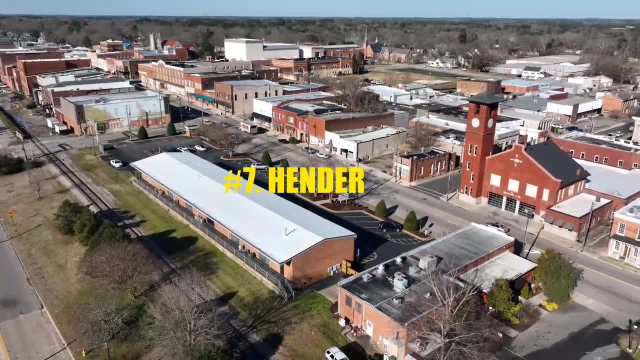 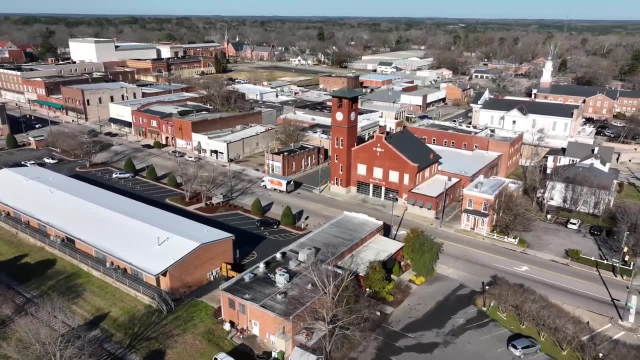 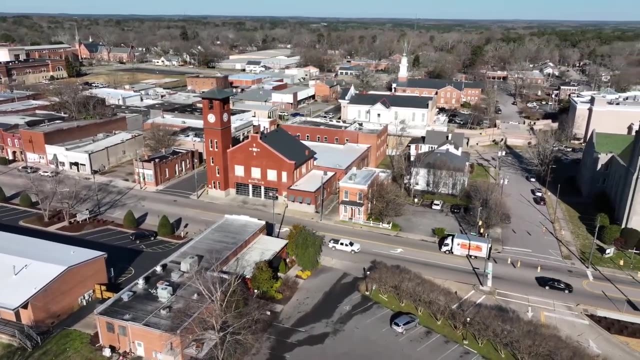 Number 7. Henderson- Just 40 minutes north of Raleigh, Henderson is a perfect representation of small-town Americana. Its effort to preserve its rich historical past has fueled its prosperity in modern times, with residents claiming the town is becoming an increasingly lovely place to live. 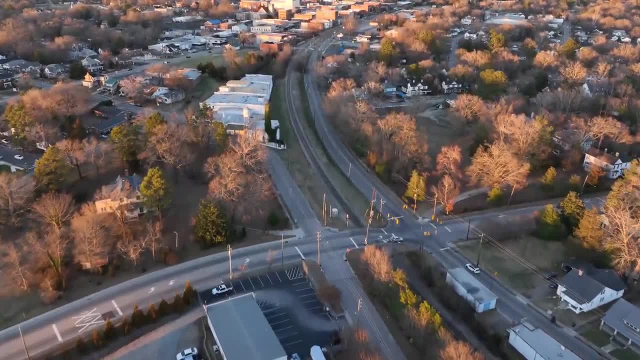 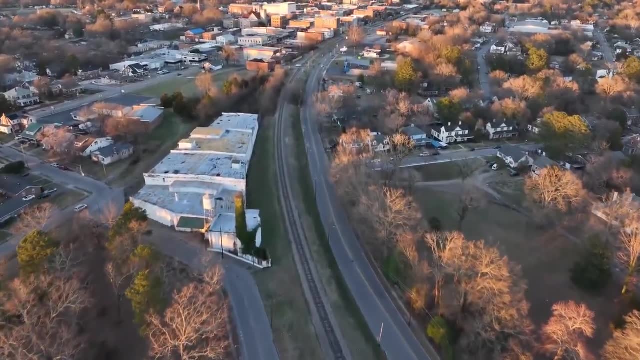 Its proximity to the Blue Ridge Mountains provides some of the best hiking, camping, biking and horseback riding in the state and, unlike some of the other small towns on this list, Henderson's culinary scene goes far beyond fast food. Like all towns, there are nice. 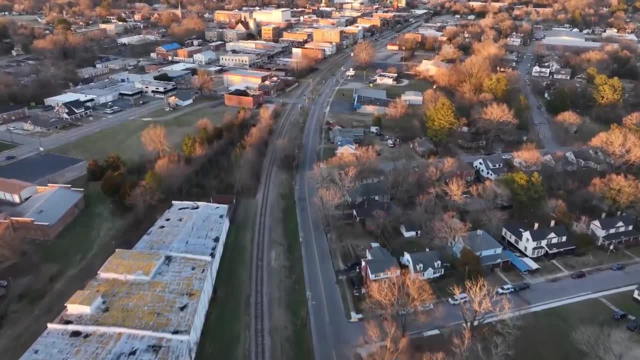 and not-so-nice parts of Henderson For young professionals or retirees looking to save some cash. you won't find a lower cost of living north of Raleigh Number 7.. Henderson is one of the most popular cities in the United States. It is home to the 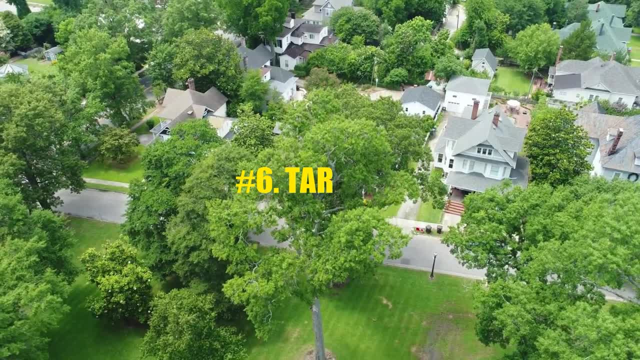 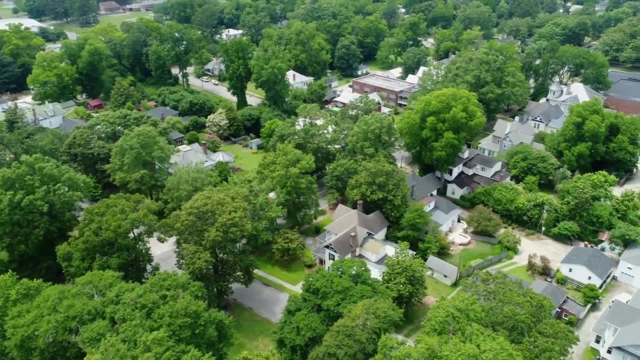 United States and is one of the most popular cities in the United States, Number 6. Tarboro. Founded in 1760 on the bank of the Tar River, Tarboro is North Carolina's oldest town. Despite its age, Tarboro has become a haven for young families and outdoor enthusiasts hoping to 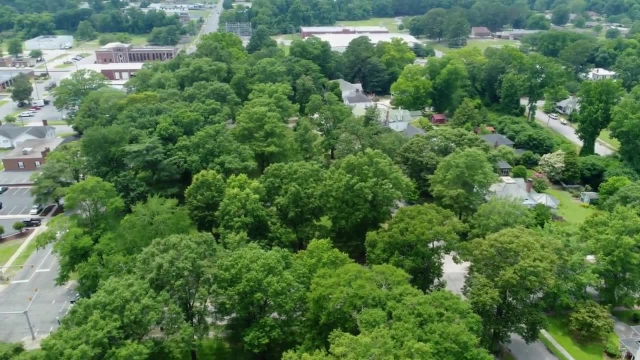 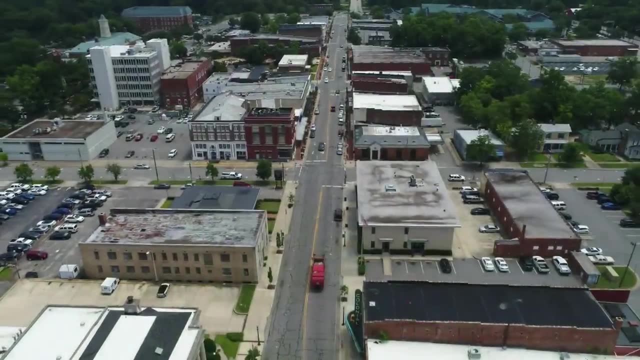 stretch their money further. The town is particularly well-known for its historic churches and 15-acre Town Common, the second-oldest one remaining in the United States. There's plenty to enjoy around the Common. ride your bike down one of the city's many cycling. 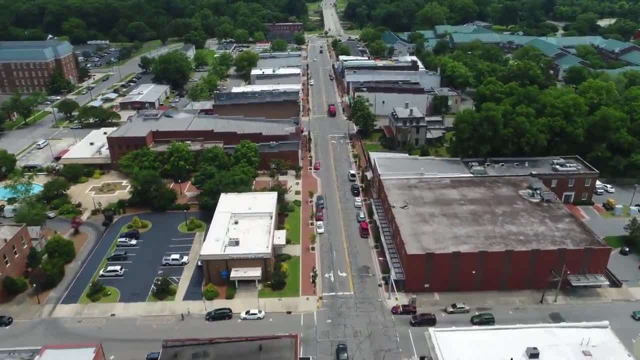 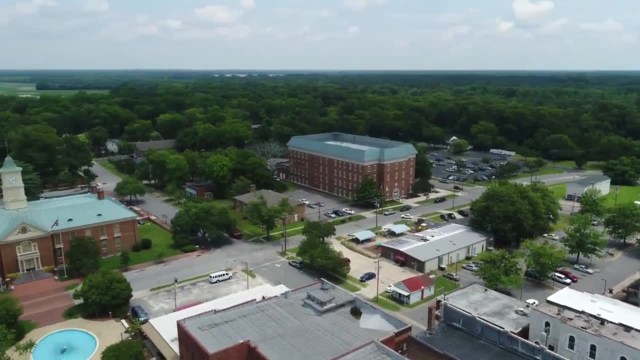 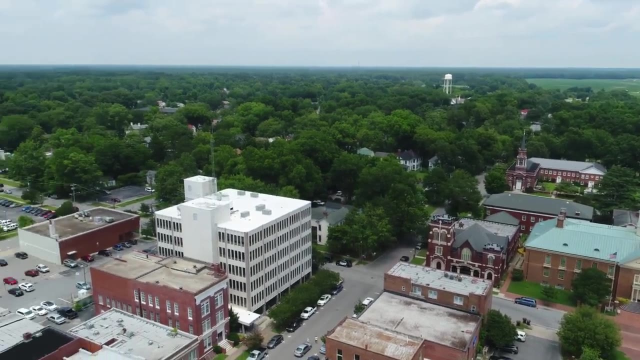 routes, plan a fishing trip out on the Tar, or enjoy a book and a picnic under the town's sweeping oaks. Over the past few years, Tarboro has welcomed three major manufacturing and distribution centers to its local economy, creating over 1,000 new jobs in the area. While Tarboro has historically been 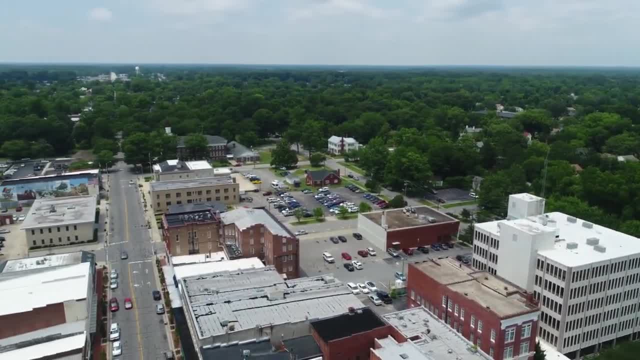 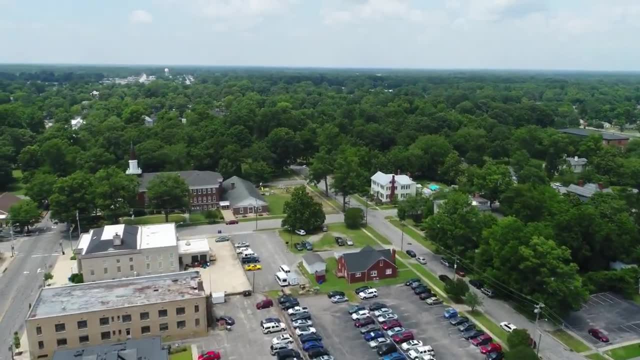 a lower-income town. its median household income has increased an astounding 38.6% since 2019.. But despite the spike in income, home and rent prices have remained some of the lowest in the state Number 5.. Roanoke Rapids. 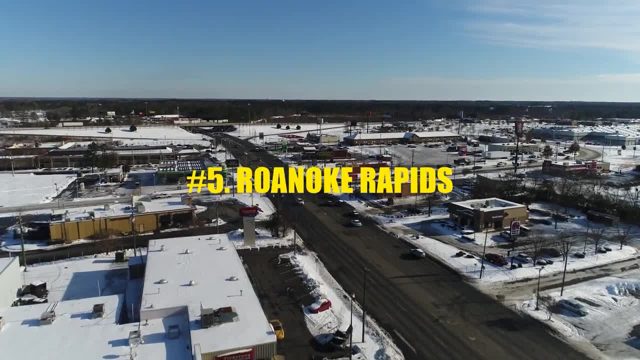 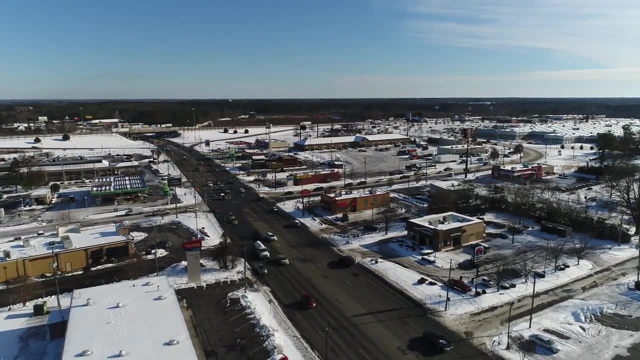 Nestled on the banks of the pristine Roanoke River, historic Roanoke Rapids boasts small-town traditions while showcasing new and exciting attractions and events. With one of the highest median incomes on the list, you'll have more to spend on the city's. 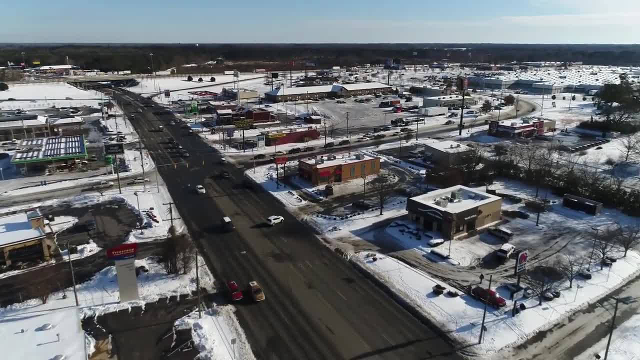 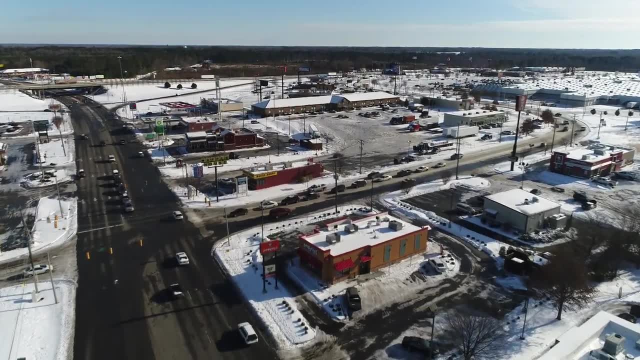 main draws. catch a show at Roanoke Rapids Theatre, indulge at Hagerty's Steakhouse or spend a leisurely afternoon touring the local art galleries. The city also offers a plethora of outdoor adventures. You'll also get a chance to explore the city's historic parks and parks. 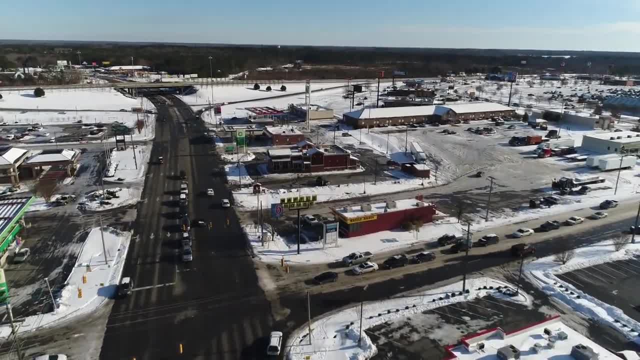 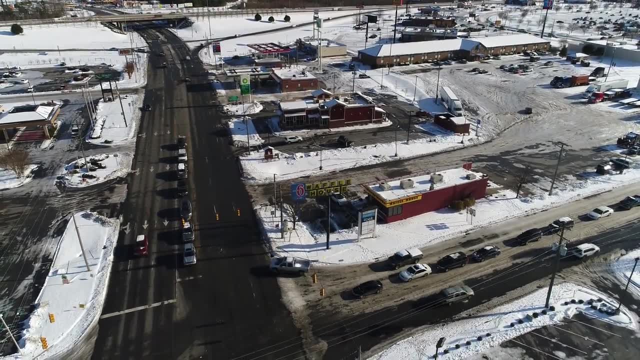 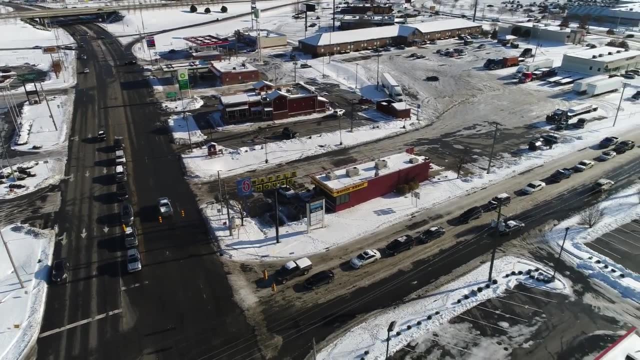 such as kayaking and hiking along the river. Roanoke Rapids is home to Westrock Paper & Packaging Mill, the town's largest employer. That said, there aren't many career opportunities outside of manufacturing, However, if you're working remotely or are a recent retiree drawn to a 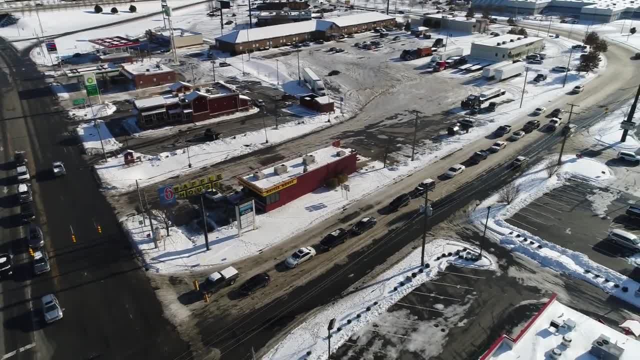 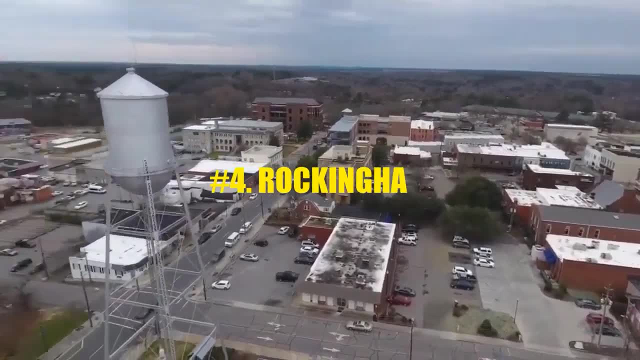 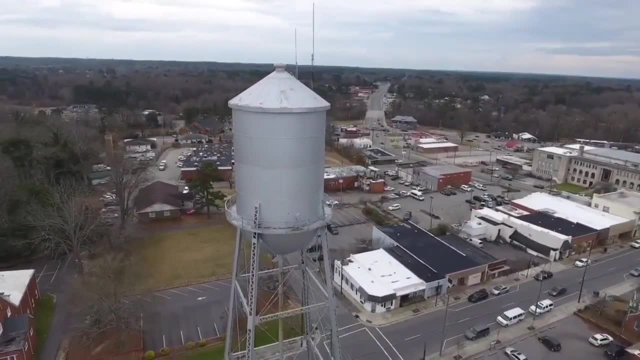 slow-paced routine, tight-knit community and low-cost lifestyle. consider checking out Roanoke Rapids, Number 4. Rockingham: With less than 10,000 residents, Rockingham is a small city to make the list of cheapest places to live in North Carolina, But don't let its size 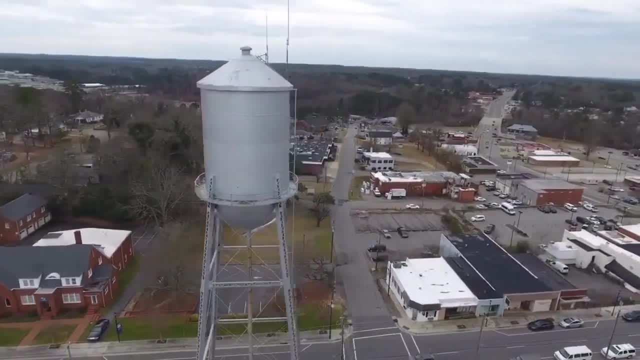 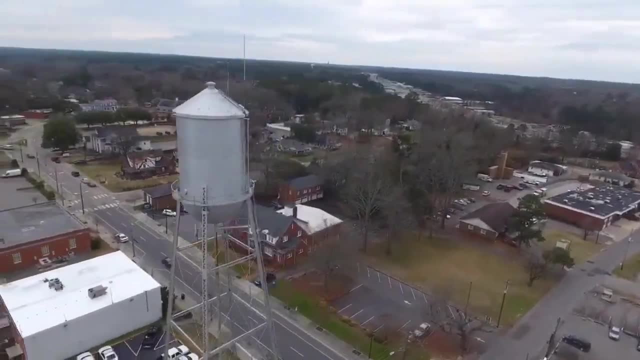 fool you—Rockingham is jam-packed with outdoor activities and events For wildlife enthusiasts. fishing and hunting at Sandhills, Game Land and Blewett Falls will keep you busy all year round. The city is also home to the famous Rockingham Dragway, the North Carolina Zoo. and the prestigious Rockingham Golf Club, so there's something everyone can enjoy If you're looking to keep bills as low as possible. Rockingham ranks number one for a $14,000 dollar rent, number two for cheapest home prices and number eight for the lowest cost of living. overall And with a newly redeveloped downtown area, you won't want to miss out on the opportunity to call this up-and-coming small-town home Number 3. Lumberton- Located in North Carolina's serene Inner Banks region, Lumberton rests on the edge of the Lumber. 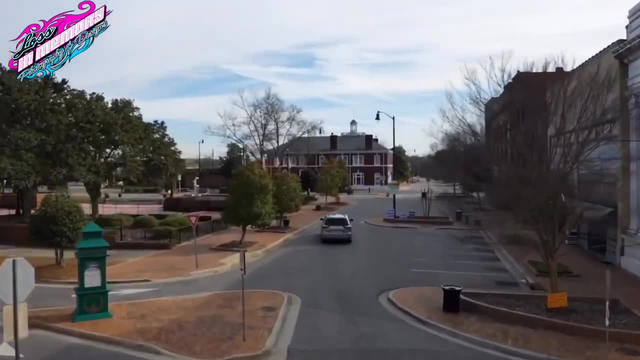 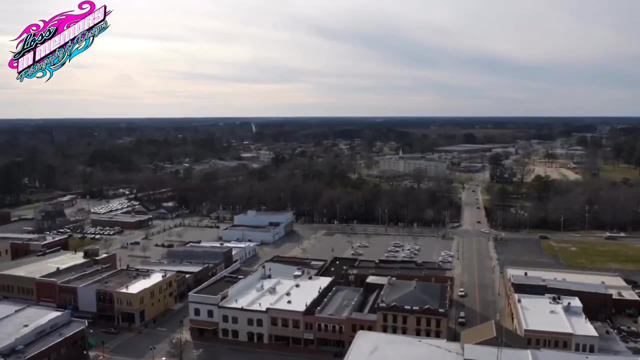 River and was an important shipping point for—you guessed it—lumber. But despite its economic namesake, this historical town is still one of the most popular places to live in North Carolina. Lumberton has embraced its location as the midway point between New York and Florida with 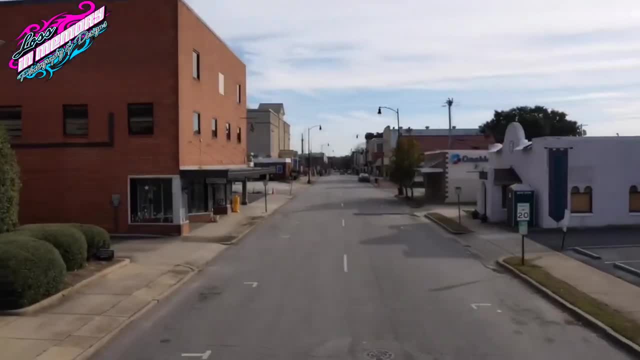 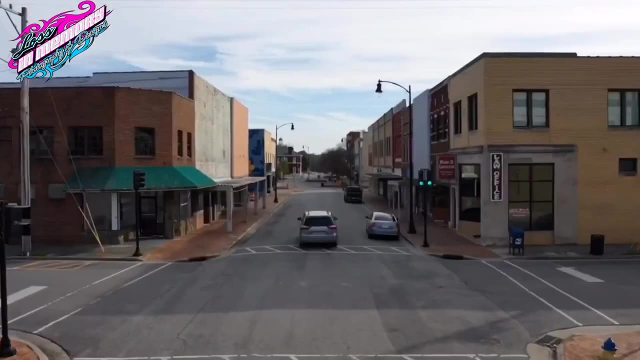 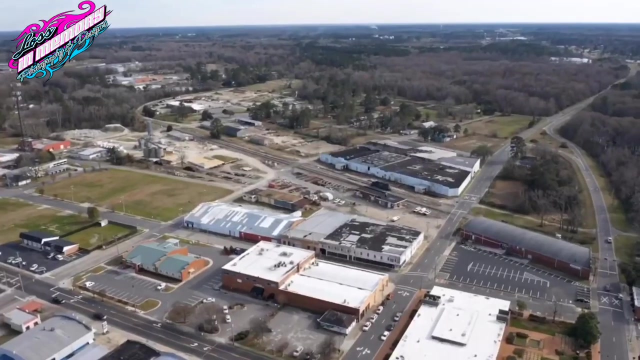 the bustling hospitality and restaurants seen- perfect for locals and those traveling through. Lumberton is also home to North Carolina's first certified retirement community, which hosts a range of convenient amenities, services and engaging opportunities for retirees. With some of the state's lowest rent home prices and property tax rates, you'll be able to live a 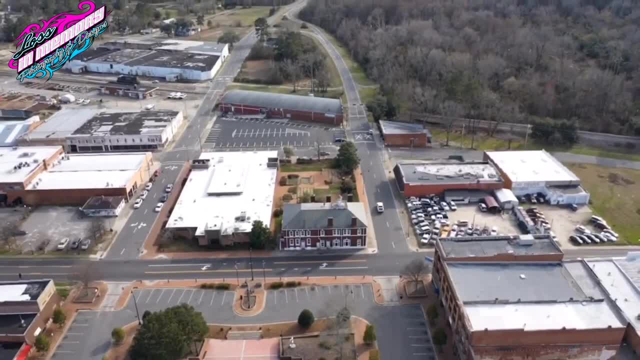 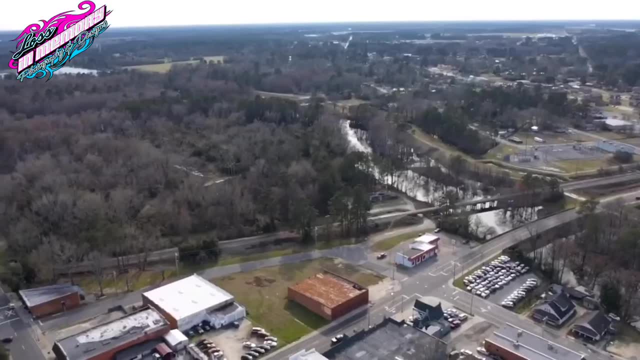 low-cost lifestyle without compromising on dining options, outdoor activities or a view of the river. If you're looking for a healthy dose of Southern hospitality and breathtaking landscapes, you'll feel right at home in Lumberton, Number 2. Laurenburg. 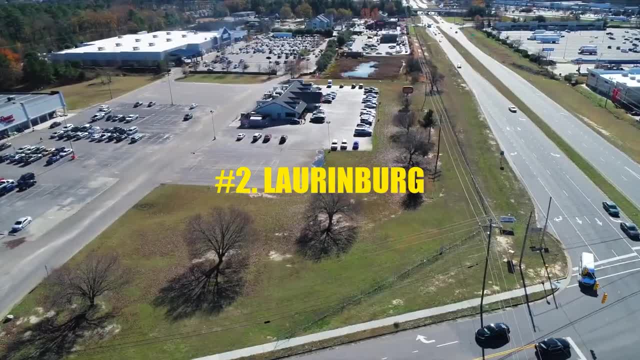 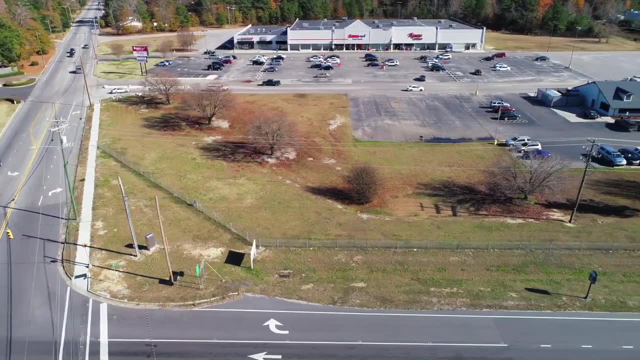 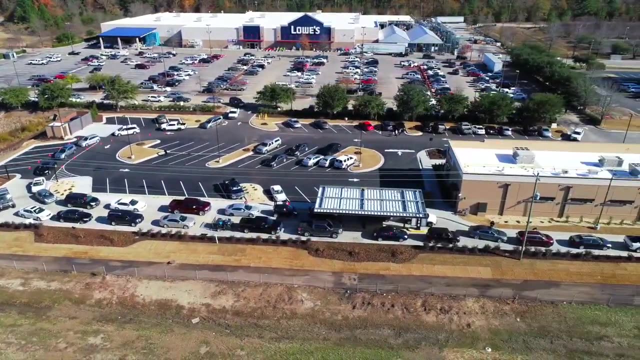 Just 43 miles west of Fayetteville, Laurenburg is a convenient location for young professionals or college students looking for a laid-back lifestyle with modern amenities and plenty of exciting things to do. Laurenburg still stays true to its agricultural roots, but the city has become a progressive business and cultural center within Scotland County. 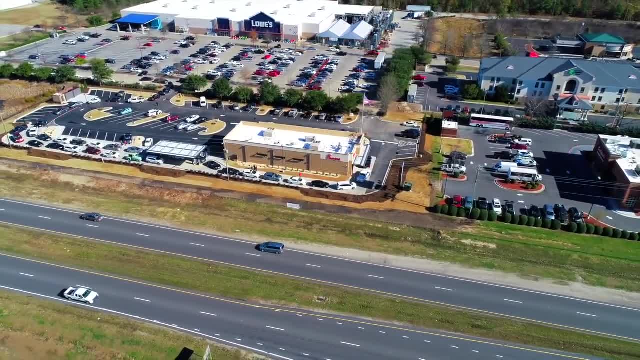 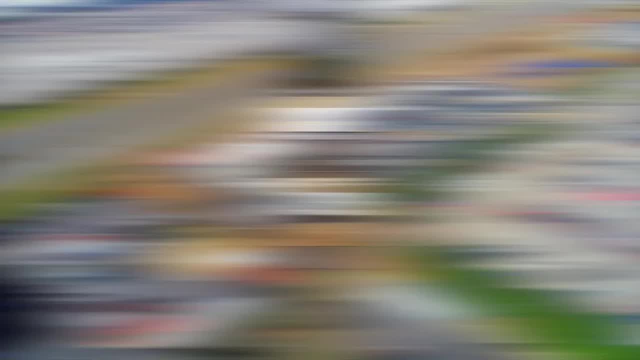 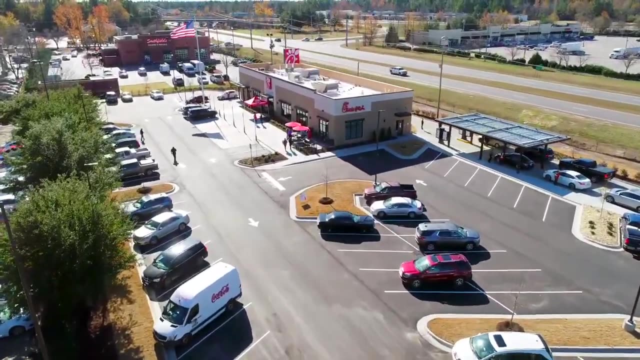 with a vibrant art scene, year-round festivals, progressive community services and close proximity to big city attractions, beaches and mountains. The 10,000 students attending St Andrews University, just south of Laurenburg, have played a vital role in bringing the city to life. This three-time All-America City Award winner ranks: number one for cheapest median home prices in North Carolina and holds the lowest cost of living rate, at 29.9 percent below the national average. That said, you'll be able to get an impressive bang for your buck in this town beneath the oaks, Number 1. Eden. Eden, a quaint little city located where the Dan and Smith Rivers meet, tops the chart as the cheapest place to live in North Carolina. Home to an energetic, historical downtown district, ample hiking trails, grade-A fishing holes and impressive family-friendly parks, Eden exudes small-town. 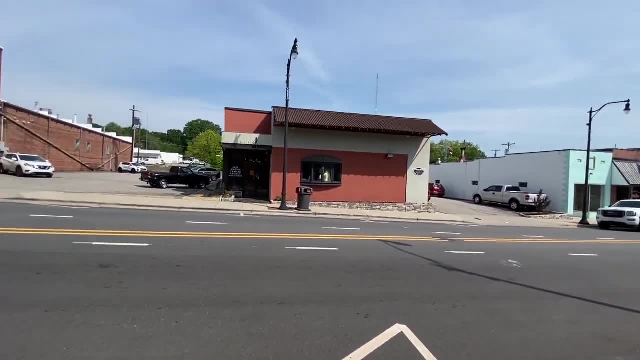 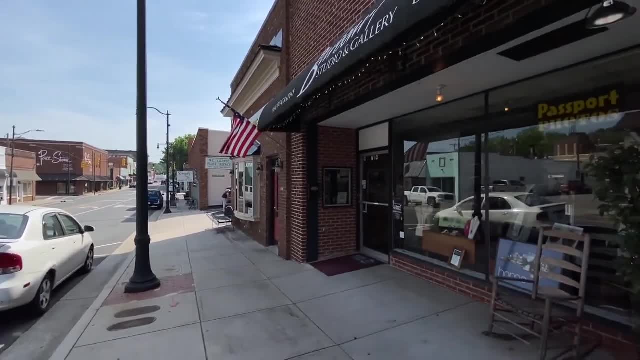 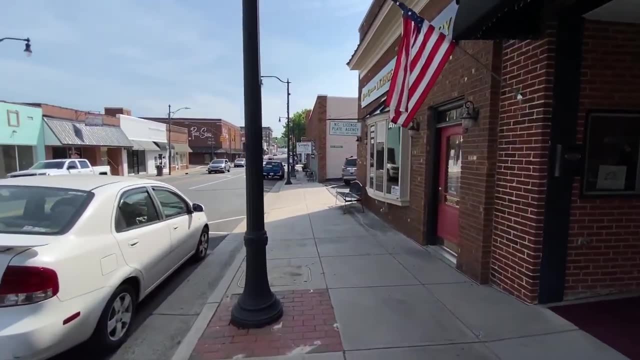 cost of living is $20,000 per month. The cost of living is $20,000 per month. The cost of living is $27.9 percent cheaper than the national average, making it the perfect place to comfortably raise a family or take some time getting lost in the great outdoors. You could spend a day exploring the nature trails. 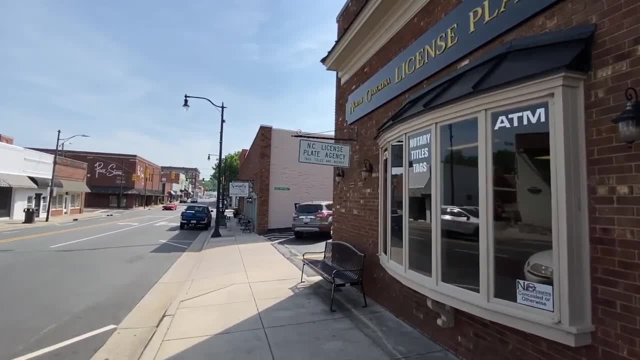 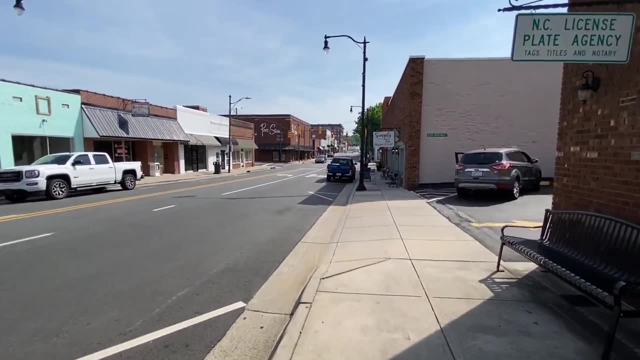 and settling in for a casual picnic at Freedom Park, followed by a pit stop at Reynolds Brewery and ending your day with popcorn and a show at Eden's own drive-in theater—all for less than $20.. So which is your favorite places among the top 10 most affordable places to live in North Carolina? 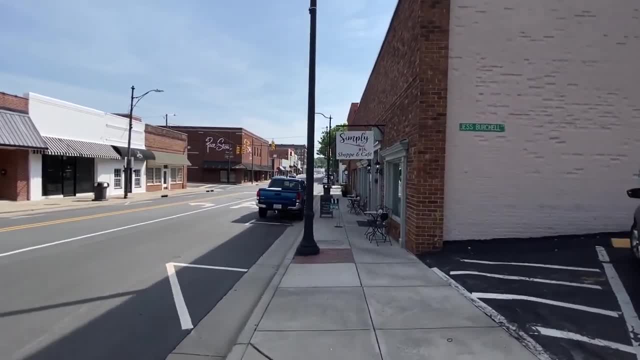 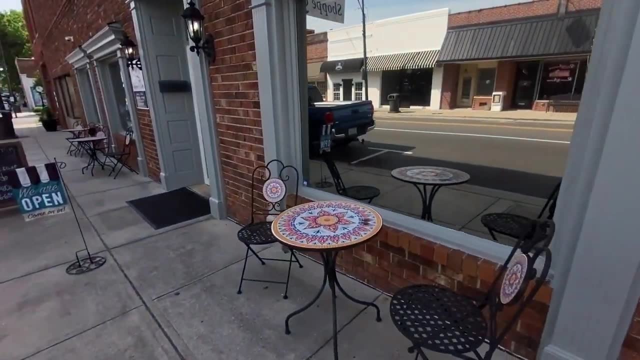 Well, that's all we have for you today. Thanks for watching. Well, that's all we have for you today. Thanks for watching. If you enjoyed the content of this video, click the subscribe button so you can receive more content like this. Post your favorite places among the top 10 most affordable places to live. 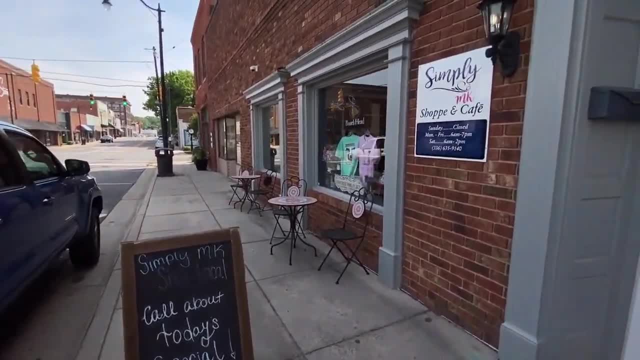 in North Carolina in the comments below. I'd love to read them and I'm sure others would too.